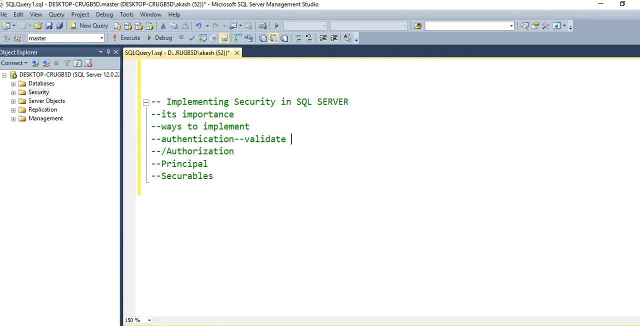 of user. in a very layman language and to remember in simple terms, it's just validate the identity of user. let's say: if you enter into a movie hall, you have a ticket. right, that ticket is explains the validity of your user. okay, you have taken a ticket, you are the valid user, you can. 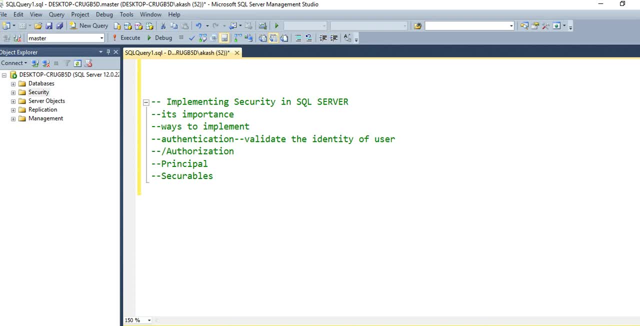 enter into the cinema hall. so, in the similar manner, authentication validates the identity of user, whether the particular user is the correct one, or the right one, or the valid one to connect to the sql server. so that explains the authentication. okay now authentication can be of different types. it can be a window authentication, form authentication, password authentication. so 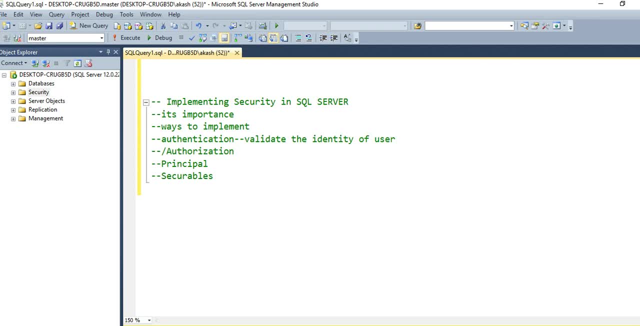 these are the. the are the types of the authentication. if you can see on my screen here. let me disconnect it. and and now suppose I wanted to connect to the sequel server. so to connect to the sequel server I have to be validate user. I have to be valid user. to connect it, let me click on the database engine and if you, 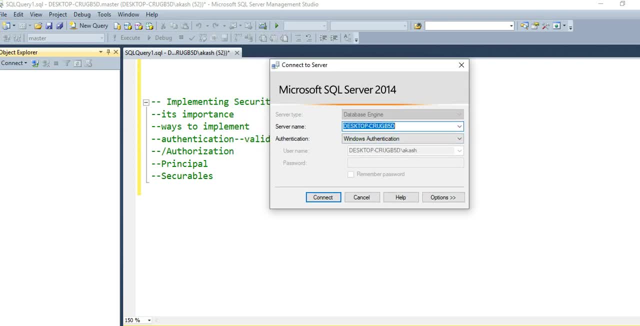 can see here. this is the server name. okay, and authentication: if you can see here, I have been provided two types of the authentication. two options are there: window authentication and server sequel- server authentication. in window authentication, basically, if you can see, username and password is hidden. why? because when I log into this operating system, I have been provided. 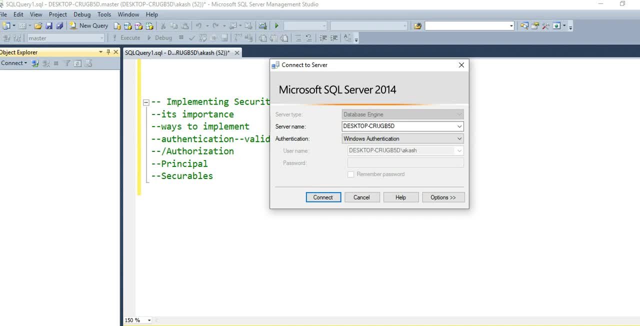 the username and password. that username password is been stored in active directory, right that? so in window authentication mode, if you selected this, what sequel server internally will pick up the username, your window username and password from that active directory and validate it that you are the right person which is connecting to the sequel. 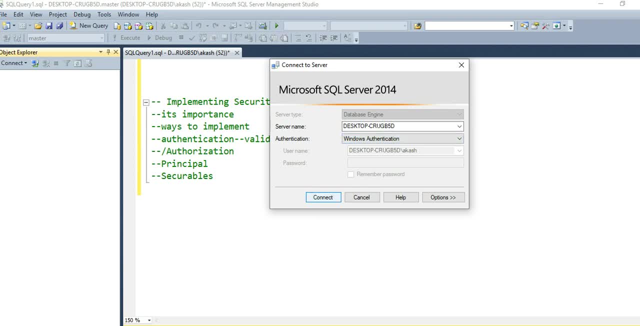 server? if it is, then it will allow you to connect to sequel server. okay, so if I connect it to this, if I click on this connect button, I will be able to connect to the sequel server. now, if you have another option- sequel server authentication- even microsoft will recommend you to connect. 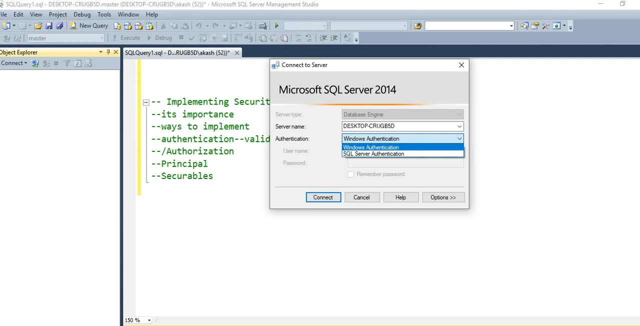 to the window authentication. but, just in case, in some of the scenarios you need the sql server authentication or you need to provide your credentials to connect to the sql server. you do not need your window username and password. so in that case you can use the sql server authentication. you can select this mode and you can provide your login and. 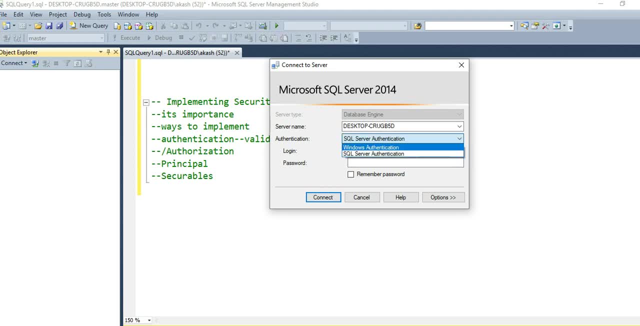 password and will connect to so and this mode. when now the question arises when this mode will be, when this mode will be selected at the time of the installing the sql server instance, when you are installing the sql server on your system. at that time you have, you have been provided two. 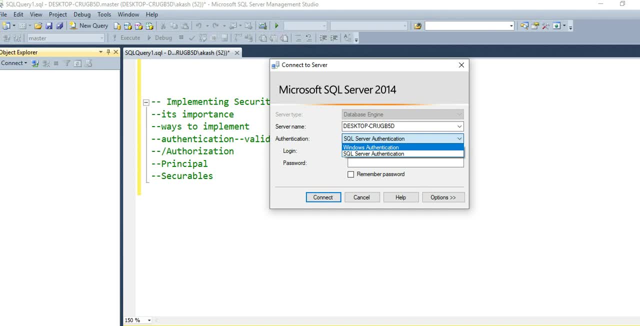 options: whether you want to install the sql server with window authentication or the mix mode. okay, if you select the window authentication, then by default, when you try to click on this, connect to the sql server. you will be able. this window. okay, you. and if you have chosen the mixed mode, then 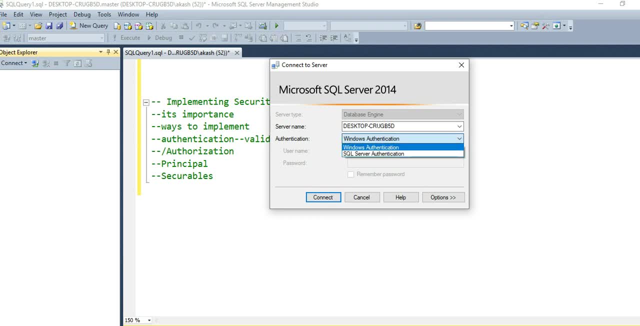 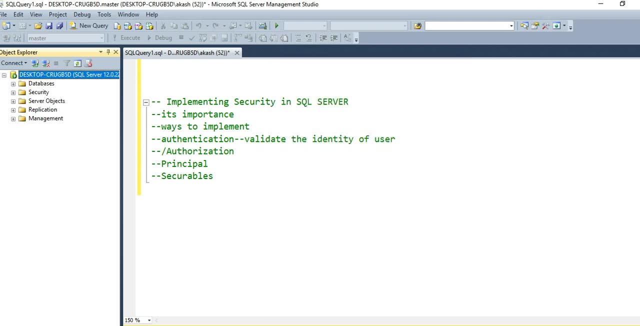 you have been able. you will be able to connect to both in both ways: in window authentication as well in sql server authentication. so as of now i'll connect to as a window authentication. so i hope that you clearly understand what is authentication. now there is one more thing. once the user will be 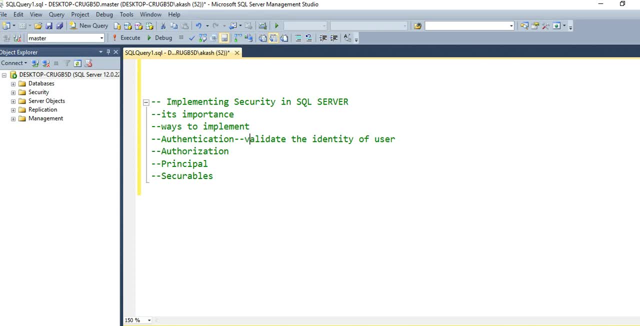 uh validate and it's allowed to connect to the sql server now in uh date in sql server instance, in particular sql server instance. this is the once in uh instance. you can have as many of instances, so that's why i'll i'm saying it as a sql server instance now in this instance. 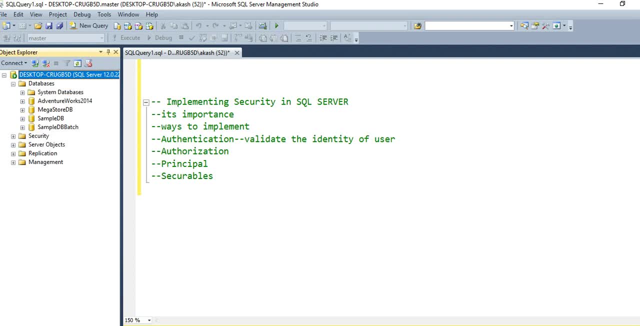 you have many databases, you have securities, you have objects, you have server level objects. so what, basically, which database this user is allowed to see? let's suppose i have this time i have four databases. okay, uh, whether i'll be able to see all the databases or to perform any queries on the 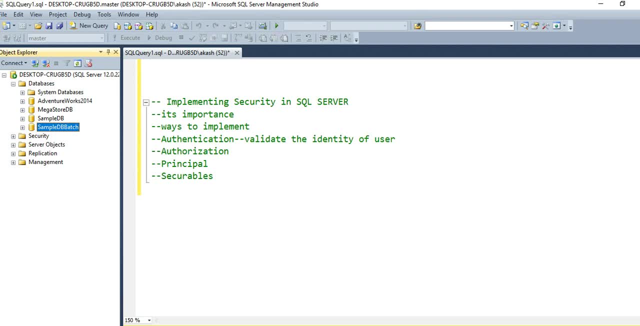 database and what type of the roles i have been given to see the data, or i'll be able to see only two databases out of four databases that privilege will be granted by will be given by authorization. authorization means: uh, what authority? uh what things? or you are authorized to see, okay, or you can see. it's nothing but a privileges. privileges. 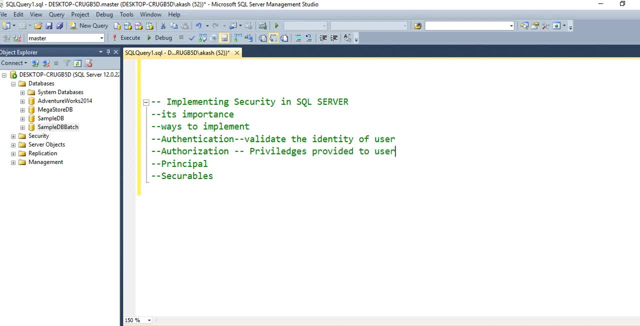 privileges provided to user. let's suppose you have entered, as uh you have entered, to the uh uh Prima Hall. okay, now you have a privilege. uh, you, you have a supreme, uh you can say golden category customer. then you have a privilege to uh sit in the top, most layer, okay. and if you have a 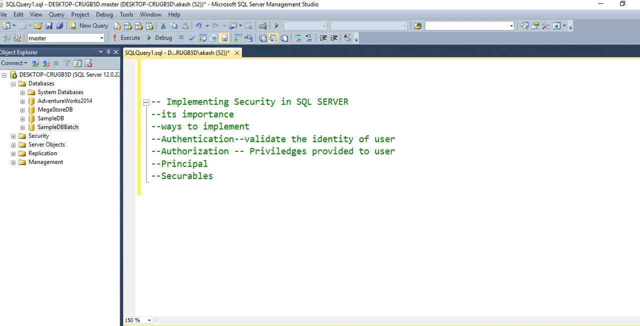 goal. if you have a silver category customer, then you have a privilege to uh up to the second row, not to the topmost row. so these are the privileges. so authorization is nothing but the privileges provided to the users. okay, then we have uh very important things uh. 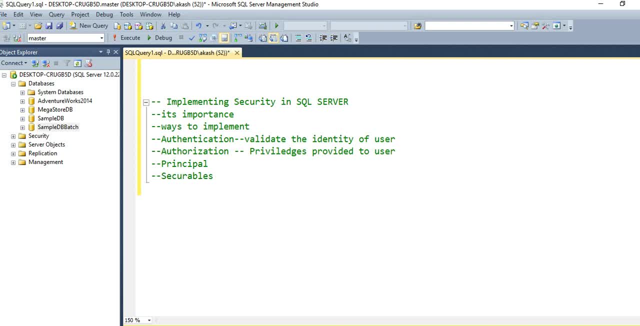 So principle? most of the users got confused by this term principle. Principle has a very wide meaning. You can say wide meaning or you can say it is an individual or collection groups. It can be an individual thing: individual users. It can be a group, set of groups, or collection or processes. It can be anything. Let me explain what it is. Principle is of two types: server level principle and database level principles. 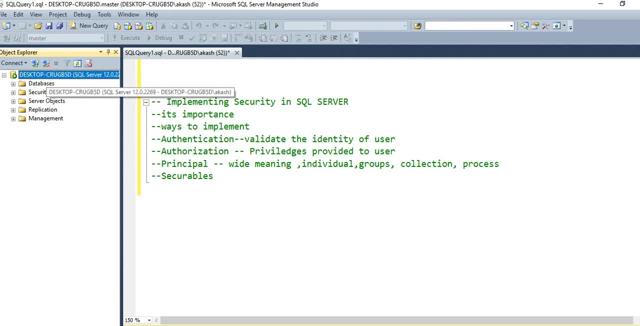 Now, if I collapse it in my SQL server instance, you can see here I have an option, I have an folder security. This security is at server level scope. We have two scopes. We will implement the security in two scopes: One at server level scopes and second is at database level scope. So this security folder explain implementing the security at server level, At this server instance level. 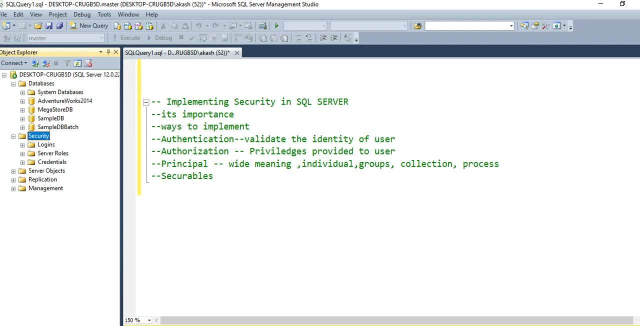 And within the server I have four databases. Let's suppose I have. I'll select AdventureWorks 2014 database it. there is one more. you can see uh option here, sorry, in this one security. so you, most of the users, got confused, or most of the persons who are learning sql server got confused by these two. 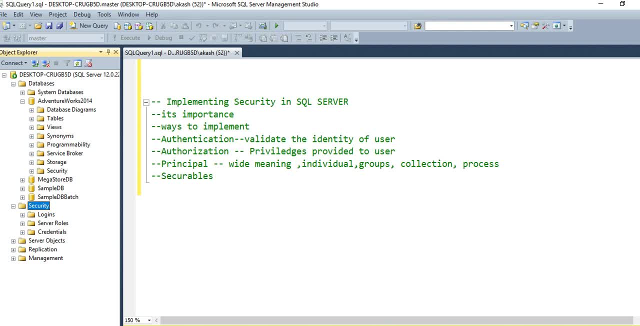 terms. uh, security folder outside and one security folder inside of the database. so this is nothing but a principle, this is a this. this security is server level principle. and the second, this security, is internally at the database level principle. so this is responsible for implementing security at server level. so in server level principle we have two things: logins and server. 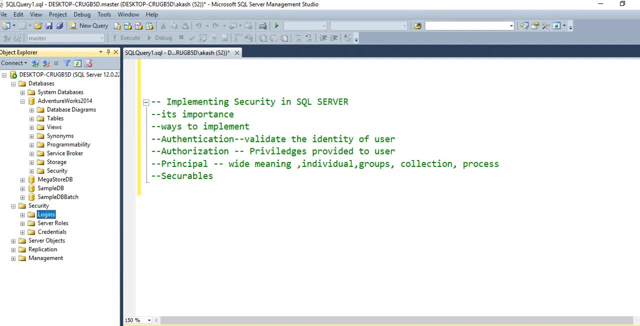 roles. okay, and in database level security, if you see, we have users, roles, schemas, keys, symmetric certificates, all these things, so i'll explain what is users and role. before that, at database level, let me explain at the server level security. first, we'll come with a login, so let me explain what is login. login and user is completely different. 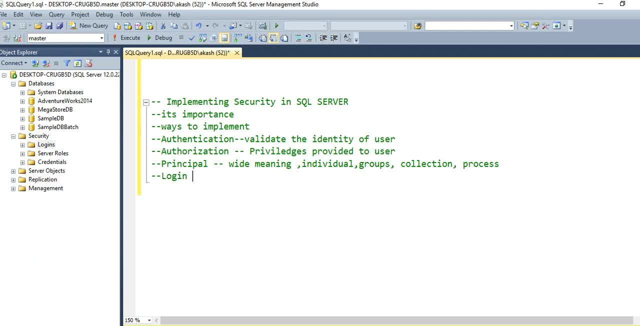 okay, let me explain you. login is something. if you want to connect to the sql server, okay, you must have one login. okay, and within a login you can have a users login is used to connect to sql server. so, if you because, why? because it's existed, the server is not connected to sql server. 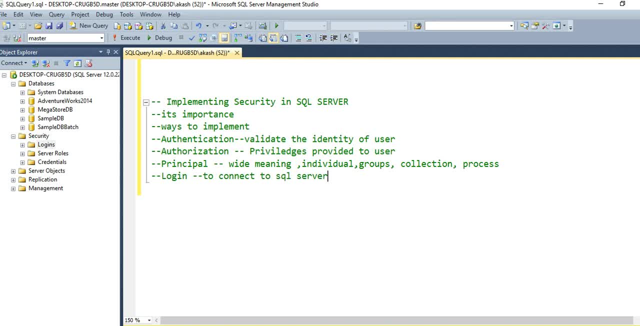 level. okay, it is not at the database level. so whenever you wanted to create, wanted to connect to the sql server, you can have a login. you must have one login, at least suppose. let me expand it and you can see here: currently i have connected to this server using login. 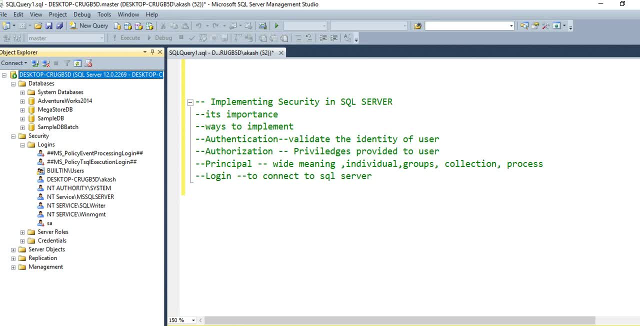 you can see this login: Akash. okay, this is my login if you mouse over it and you can see here i have connected to the sql server instance using this login. okay, so this is one of the login. okay, and if you want to connect with some other login, you can create a login. 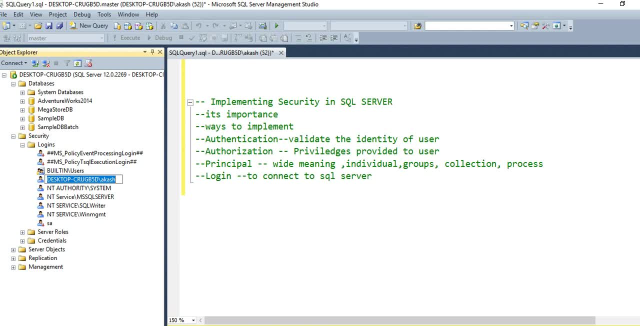 there is a t-square statements and i'll i'll show you what is the command of creating a new login and, using that login, you can give a name of the login and you, using that login, you can connect to the sql server instance. so login is nothing, but we use the logins to connect to the. 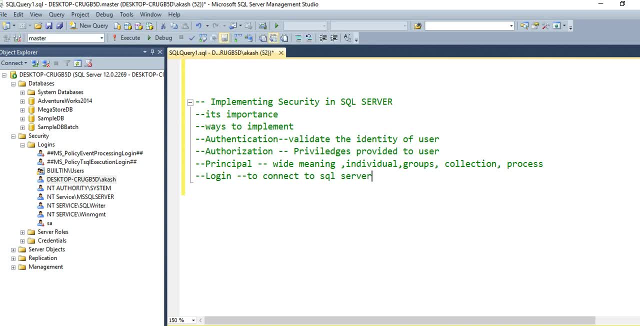 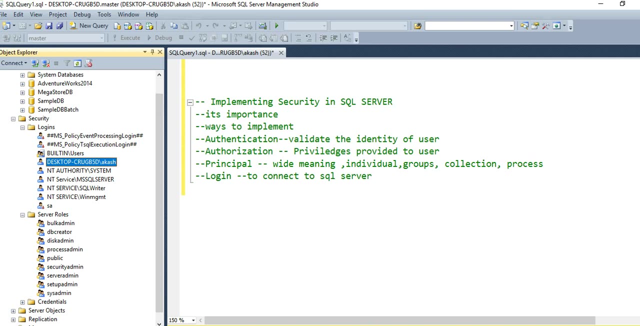 sql server. okay, now we have a server load. now server rows means uh to this particular login. what are the rows is been provided to the particular login. so uh, at a server level. so we have one, two, i guess nine server level rows, rows. you can say uh, the privileges, or we can say okay. 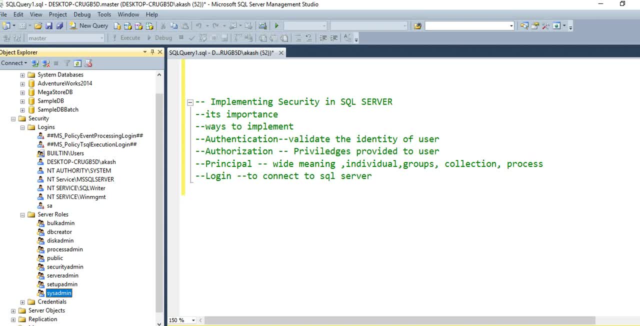 rows: uh, the number of row, number of privileges will be collection. the collection of number of privileges will be: uh, come together in one category and will be termed as a role. okay, now, bulk admin, as a name says that. i'll explain. i'll give one uh line statement of each of the 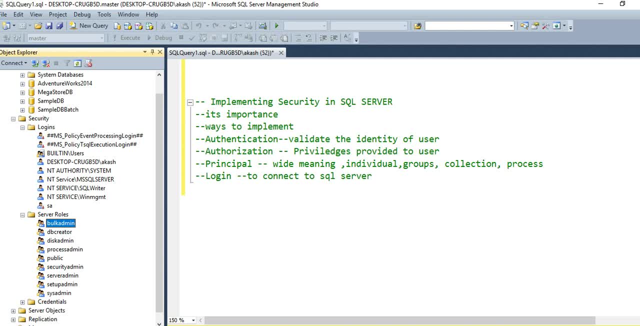 server role, bulk admin, uh server role, will say, will explain, or the member of you can say a member of bulk admin server role, will be able to execute the bulk insert statement in sql server. okay, only the users which have this role, okay, only the logins which have this role, bulk admin will be able to execute the bulk insert will be. 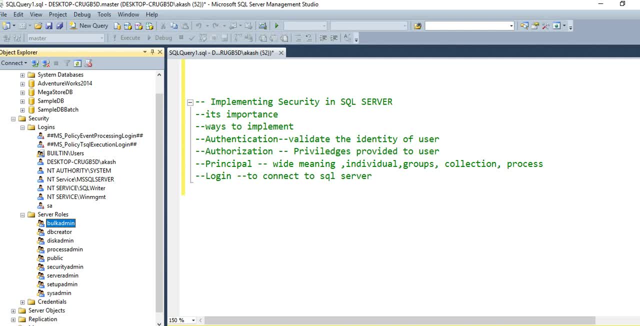 able to insert the data in bulk mode in sql server. now, second is db creator. db creator means database creator, so the member of this role will be able to create databases in this sql server instance. it will create it, will it? it can drop, it can alter the databases. then we have a disk admin role. 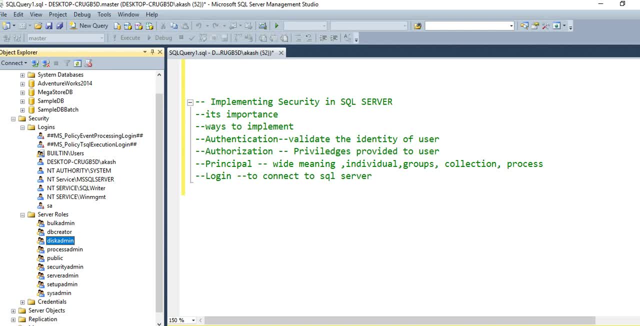 the member of this uh role. okay, then all the members will be able to create databases in this sql server instance. so the user which uh having this role will be able to manage the disk file in which the database in which the data of sql server is actually, or the data of different. 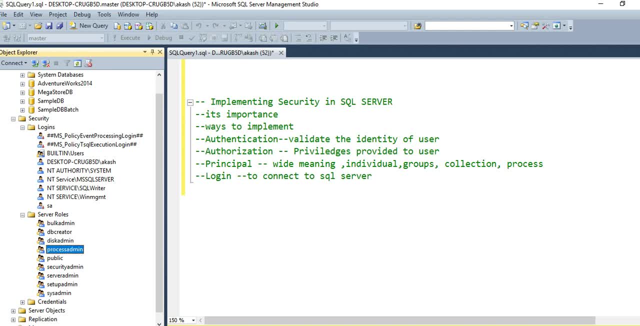 databases is actually stored. okay. then we have a process admin role. the member of this role will be able to kill any of the process which is currently running in in your particular sql server instance. then we have a public role. this is the general role and it it is by default role. 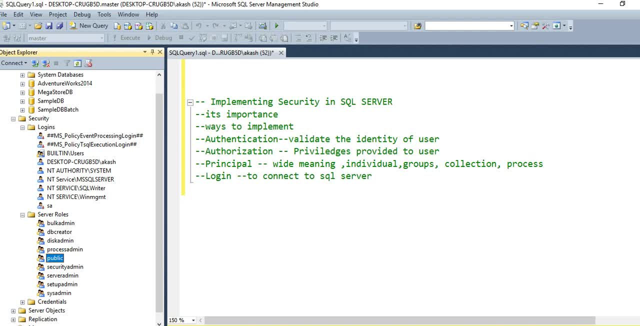 will be provided to every login which will connect to the sql server. then we have a security admin- security admin. you can say it's an administrator, it can implement or it can change the secure. it can change or administrate the security at the server level. then we have a server add server. 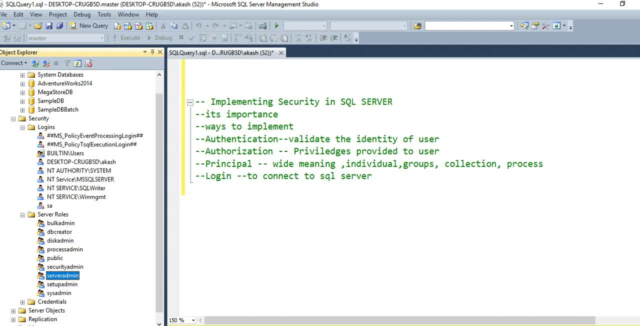 admin. this is able to this role, will be able- or the member of this role will be, will be able, to change the security at the server level. then we have a security admin, which will change the server configuration and files. okay, setup admin is basically, uh, the same. 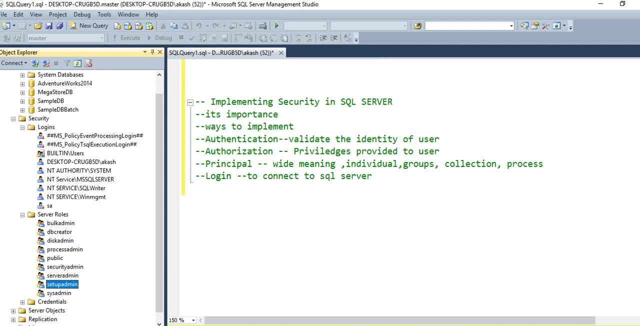 you can see it can remove or add the linked server. okay, it can set up the linked server. linked server means a server which is outside of the current server and you wanted to link two servers. so for that, uh, if you want to do that, you must have to do with the users, which is having the setup. admin. 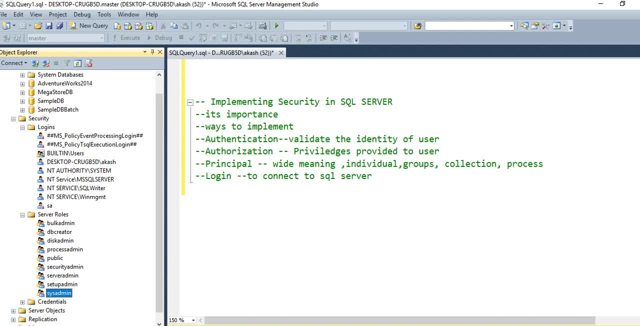 role then sysadmin. sysadmin is basically: uh, can perform any activity on the server. okay, so these are the server role roles, or we can say the server server level principle. we can say that: okay, so these are the server level security, this which has been provided by the sql server. 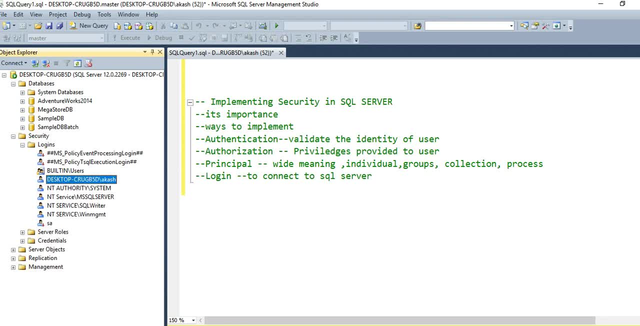 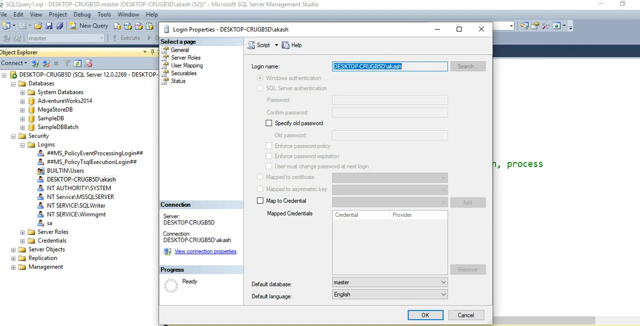 if you wanted to see like i have this login, if you wanted to see this login is having which server roles. so you need to do how you can do it. you need to open the properties of this login. when you click on this, you will find in general: uh, the name is there login name. then in second server rules: 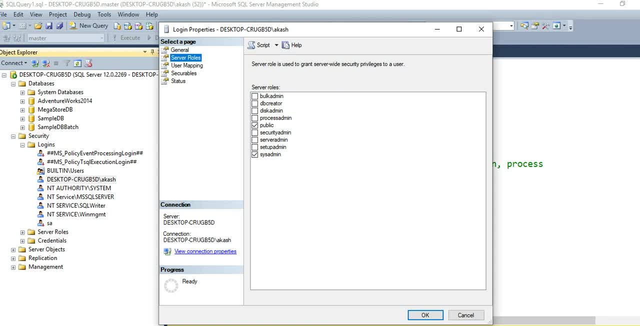 now for this particular login. you can see only two rows. server waiver rules will be provided to my login. first is public, which is by default, and second is admin. that means this login can be uh, the will be able to perform any activity on the my current sql server instance. okay, 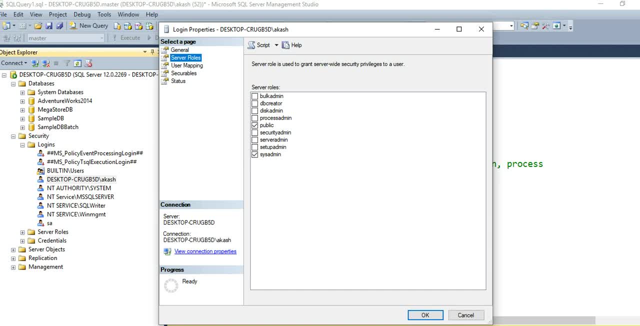 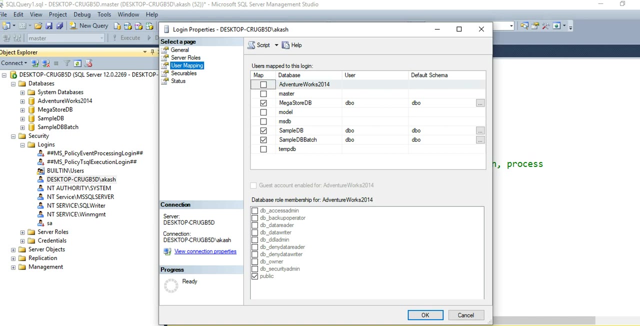 then we have a user mapping there. third option: when i user mapping means, uh, this login will be uh able to which uh databases, okay so, or it is mapped to which databases that that actually it means. so when you click on it you can see we have uh this much of databases in my sql server and my login is will be able to. 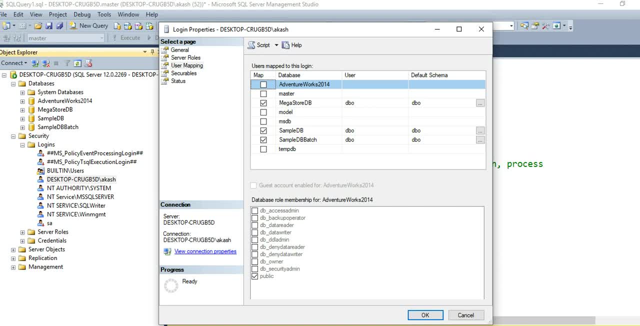 see megastore db will be able to perform. uh will be able to see megastore db sample db. sample db database. okay, so these are the databases uh, which uh in which the my login will be able to see or connect to, now for, but and if you see in the next, this database. 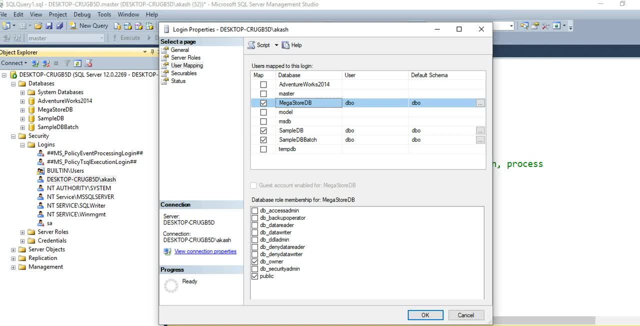 role: membership for megas2. so this will explain you that, or at database level, what actually roles you have. okay, so in megastore database i my uh login will have db on a role and public role. i uh, what i have explained earlier is a server level role. these are the database level role. 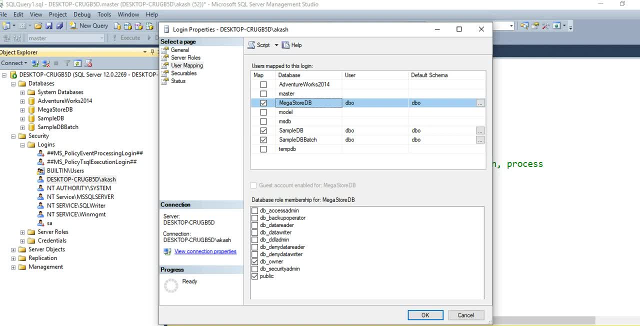 i'll explain it, but you can see here this is the db owner. so that means my user will be able to uh perform any activity- ddl commands or dmail command- on the megastore db because i have uh, because it has a honor, uh, it has ownership, it has on a role, so i'll click on it and secureable. 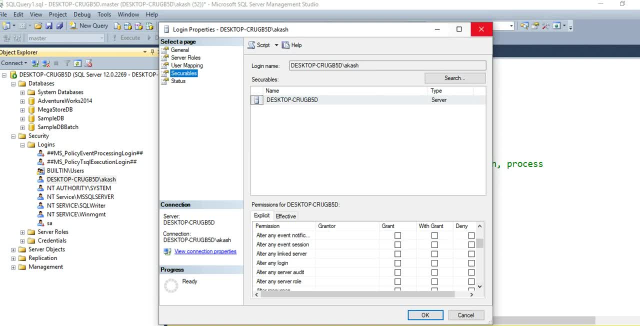 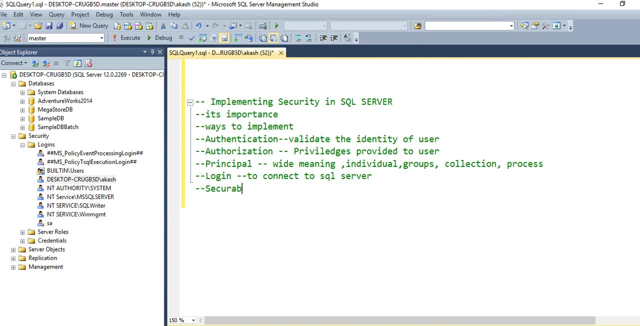 there is a permission. secureable is nothing you can say it's a permission. there is one more key term: uh, secureable variable is add, comes in in our depth. so principal is a wide meaning. you can see it's a very low level meaning it. it means in in particular database you want, but you want to. 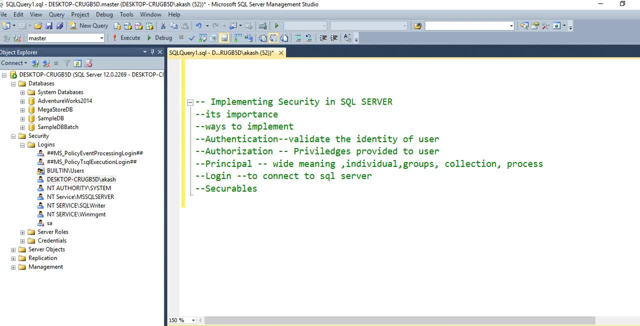 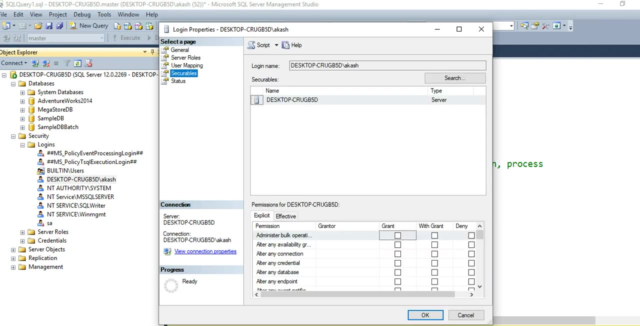 only execute you, you, you want to only read the data from particular table you don't want to delete, from delete uh, on particular data for. so in that case you can use secure- secureable. let me go to the properties of login and click on the secureable. you can see these permissions. 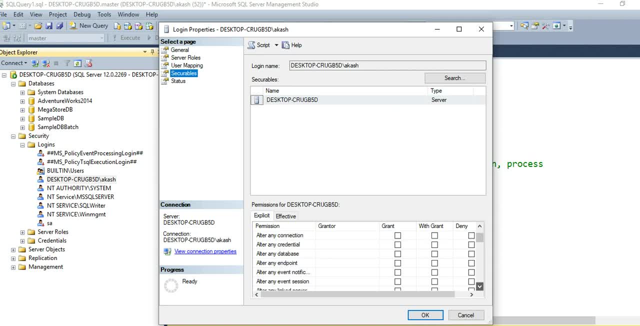 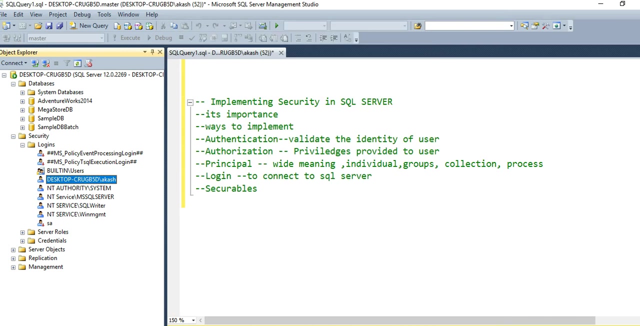 grantors. if you want to grant that permission, you can click on, it suppose, connect any database. i wanted to it to connect to database. so these are the set of permission. if you wanted to control, you can click on grant. okay, if you don't, you click on the deny. so at this level you can give the permissions. so giving 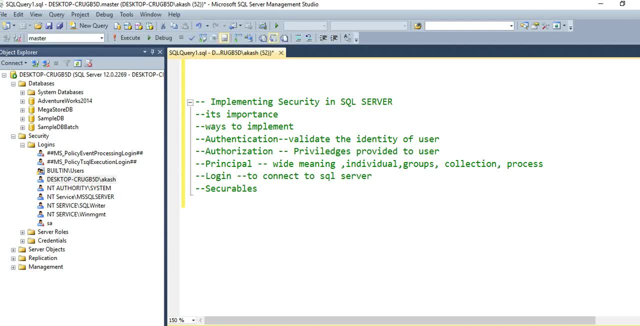 the permission is nothing but a secure level. now i'll i have explained the server level. now, at the database level, let me explain adventure work database. in security folder we have users roles. now users are what is users? so by default, if you do not have any users for your login, 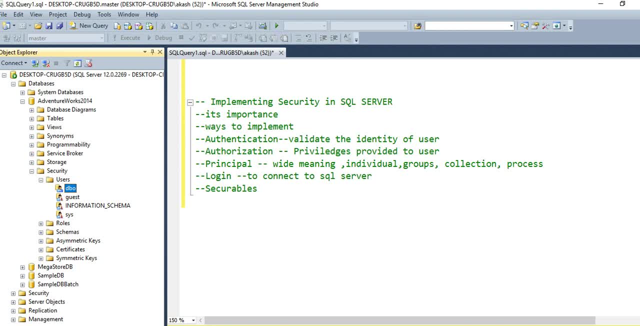 if you can see here, i do not have any other login except dbo. dbo is a default login, default user provided by sql server once you connect to the sql server using login. so when i so, this is the default user and so we can have as many of user for a particular login. okay. 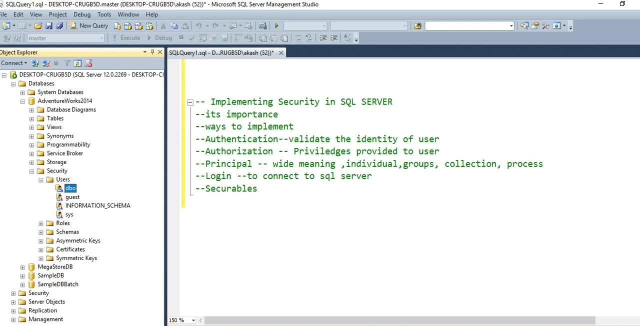 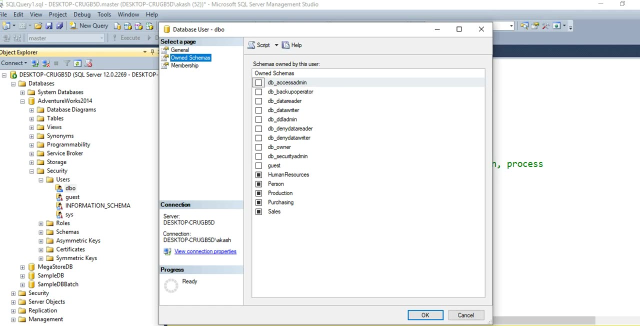 so i have a login- akash- and for akash login i can have multiple users, which is now, which is now which can be mapped to that particular login. if you go and check the properties of your users and if you see so, these are the own schemas. schemas means this user for as this. 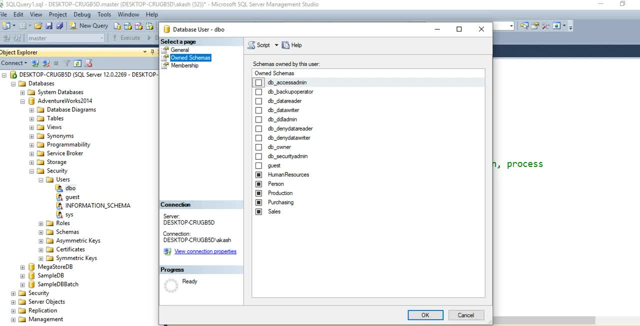 user is only for the adventure work database. so i have this many of schemas: human other than dbo schema. i have human resources, person production, purchasing, sales, so this schemas is only for dbo user can able to access it. okay, if you wanted to see what this schemas, let me open. 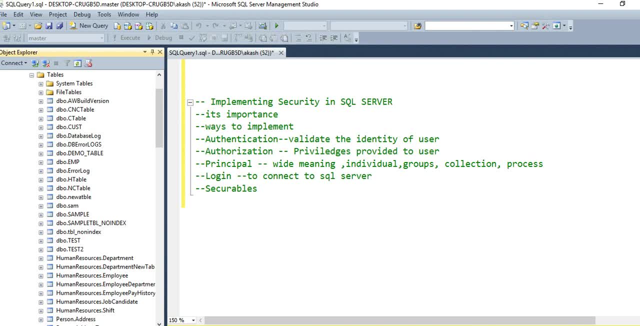 this tables of this adventure works. you can see dbo dot cnc table, dbo dot database. so what? dbo? dbo is nothing but a schema. if you see, this is the default one when you create a table and you will not provide any schema, then sql server provide the dbo dot table name and there is a custom. 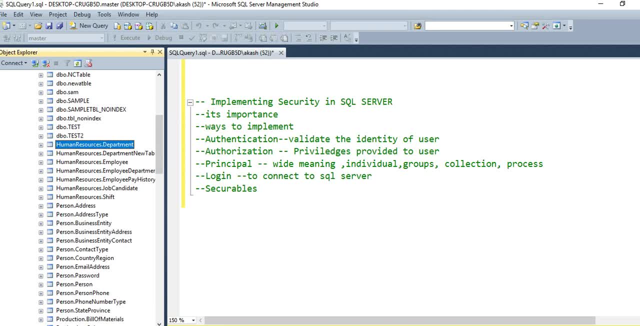 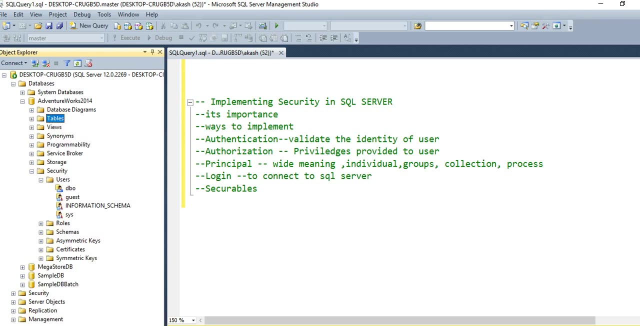 uh, if you can see human resource dot department, human resource dot dot, so this human resource is one of the schema. then we have person dot address, percent or address type, so this is another schema. so the user is having able, will be able to access all the schemas. okay, then we have a rose. rose is not. uh. now at database, we have a database. 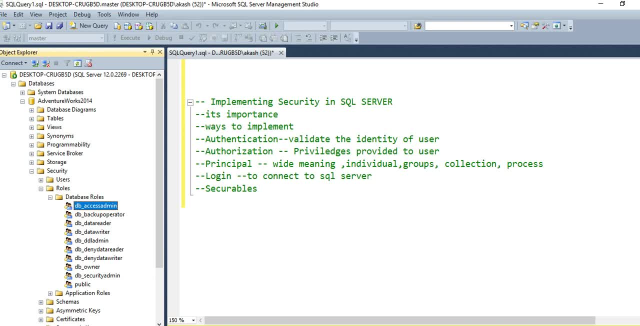 rules. let me explain it. so we have one, two, three, four, five, six, seven, eight, nine, ten, so we have ten scheme. uh, so we have one, two, three, four, five, six, seven, eight, nine, ten, so we have ten schema. uh, database level rule, so access admin. so what? uh, you can see db. uh, each of the role will be start with. 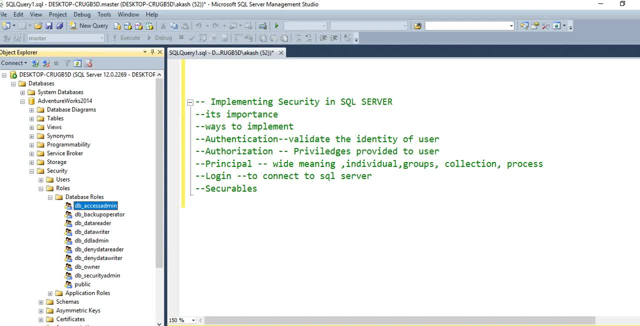 db underscore: access admin. so these are uh. access admin means it will be able to access the database it will backup. it will be able uh- the users which falls under this category, which is having this role, will be able to take the backup. uh will be able. this role data reader will be able to read. 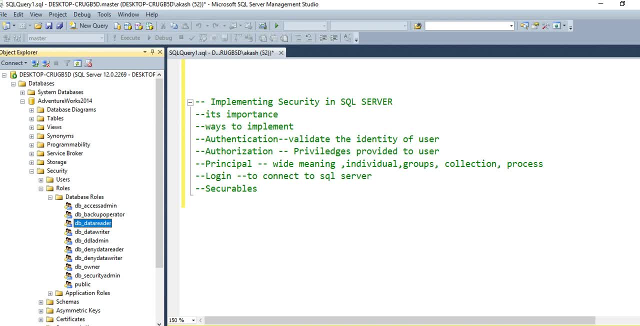 only the data within your database. it will not be able to write anything. now the user which is having this role, db data writer- will be able to write the data. okay, you will be able to insert ddl means it will perform the ddl statement. it can perform ddl statement. links alter. 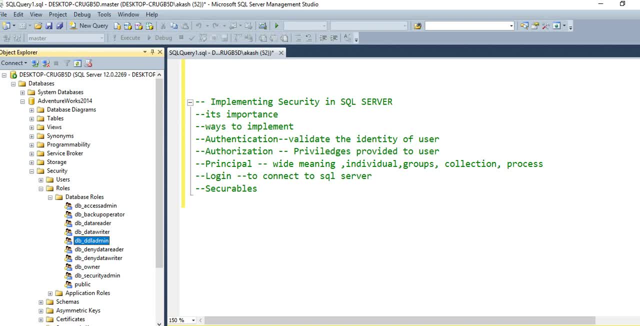 delete, alter columns or tables. okay then. deny data reader is one of the role. also, as the name suggests, it deny the reading of the data. then we have another deny data writer. it deny the uh it uh evoke or it will take your permission of writing anything in your database. then we have a db owner. 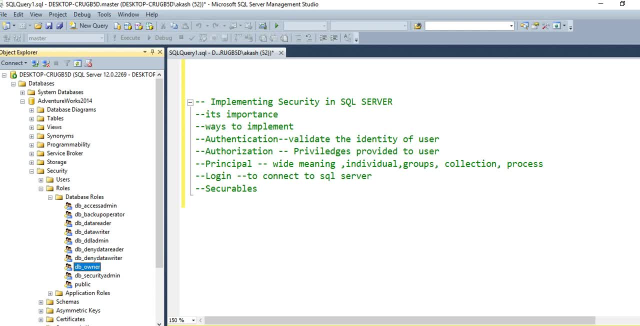 db owner means your user is having all permissions on your particular database: it can read, it can write, it can delete, it can alter the table, it can do in everything. then we have a db security admin. in db security it's implement the security and database level. then we have a public- public is. 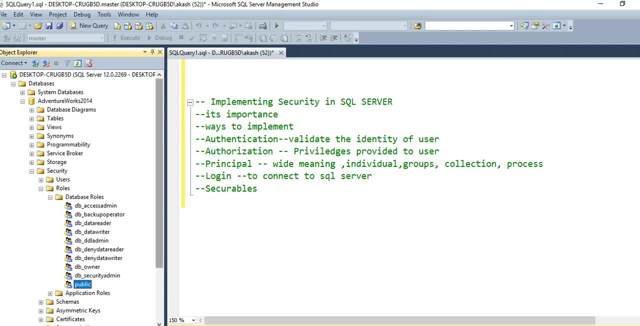 nothing but a journal database store, you can see. so i hope you understand the db security level, understand? uh, you understand what is the difference between the security at database level and security at server level. okay, and in later session i'll explain how to create a login, how to create a user and perform and provide the permissions to that particular user. and 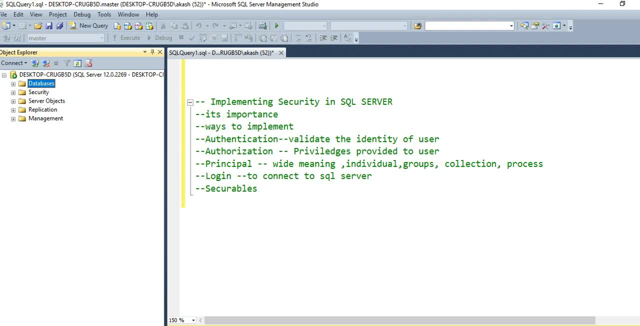 and will show you how to connect uh to the sql server instance, uh, with the which you have correct uh which you have recently created. this is a conceptual presentation, uh, in next video i'll uh i'll give the demonstration. how to create a new login, how to create a new user. 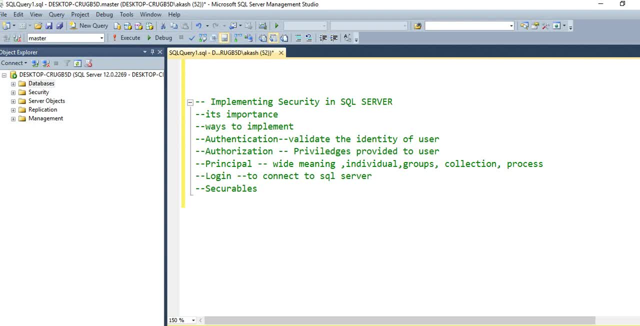 and how to perform, uh, give the grant, the permissions, or how we'll give the particular roles to the users. i hope you understand the concepts of sql server and understand the security in sql server. thank you for watching. have a nice day you.